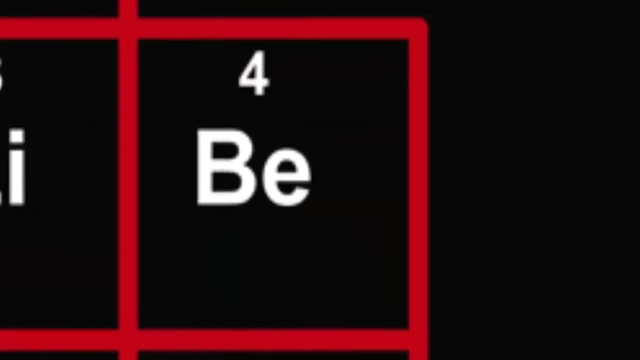 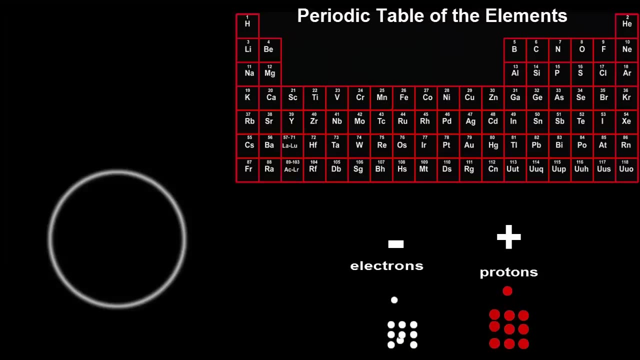 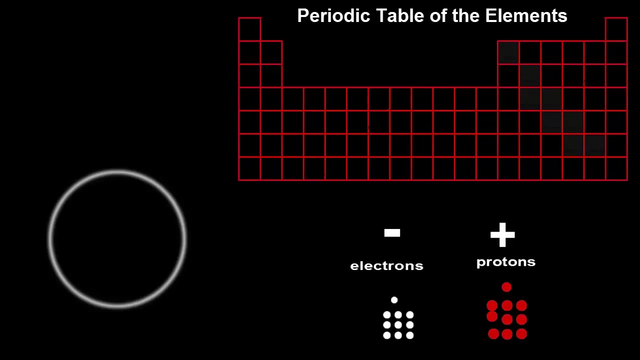 As we add more, we build elements with bigger atomic numbers. After adding 10 protons and 10 electrons, we will have neon. Now let's start with a blank periodic table and add protons and electrons. See if you can spot the connection. 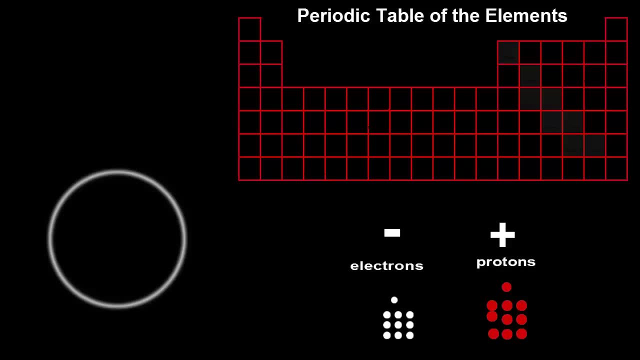 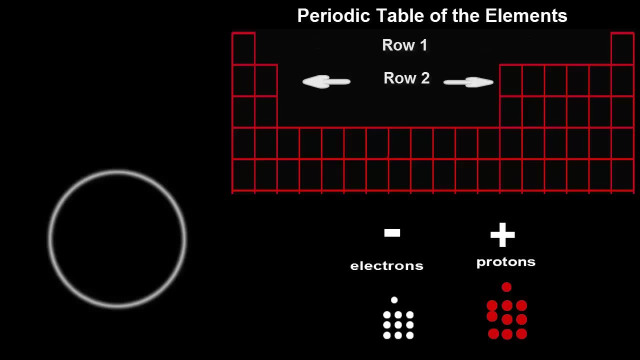 Because we're only making the first 10 elements of the periodic table. we only need the first few rows, So let's zoom in on those. We'll start from the beginning by making hydrogen again. As we make the atoms on the left, we will put them into their position in the periodic table above. 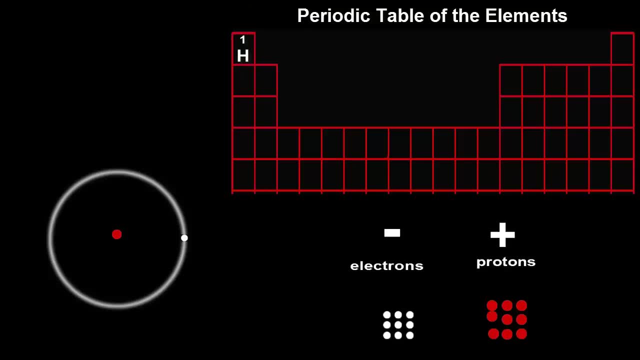 One proton and one electron makes a hydrogen atom atomic number one. Now watch the rest. If you do more resistances, you will lose this experiment. This is where brings us to the most importantbehind the discussion. today We're working on the다고영 바꿀다. 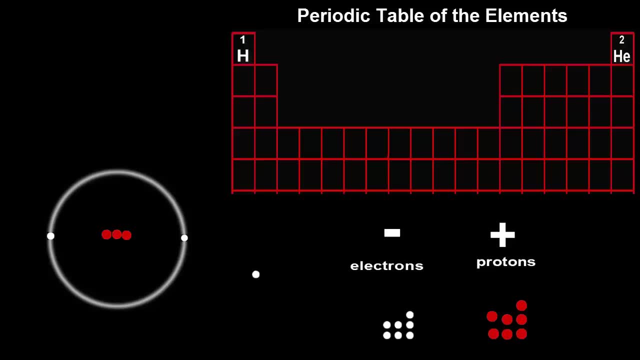 By the way, if you see this image from the race entrance that we took, the last record we forget is the one that goes down with the other ones. The one block that goes down is called an electronArchon, It's not a particular Rab. poderia 그것 diz. 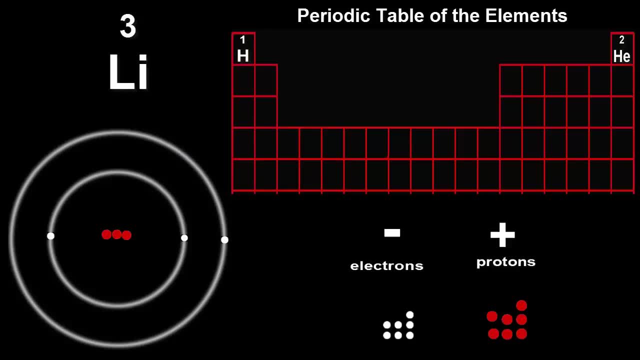 We'll be right back, We'll be right back. We'll be right back At where the protons in the nucleus show up on the periodic table. With one proton, we made the element with atomic number 1, hydrogen. With two protons in the nucleus, we made the element with atomic number 2, helium. 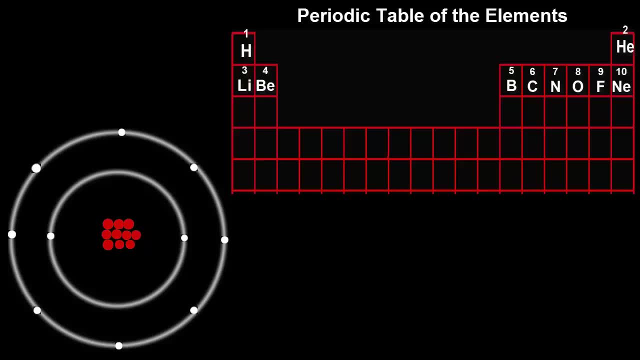 There's a simple connection between these numbers. They're always the same. The atomic number of an element is equal to the number of protons in the nucleus. You can't get much simpler than that. Now let's look at where the electrons in their shells. 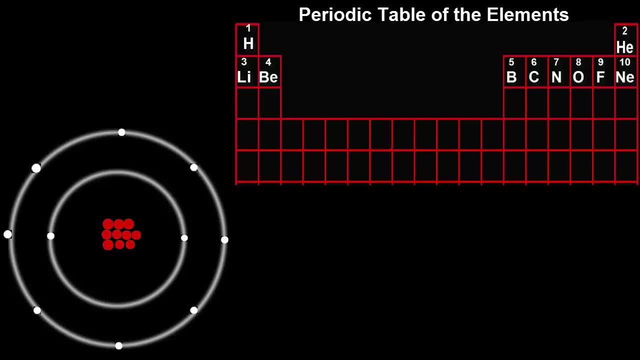 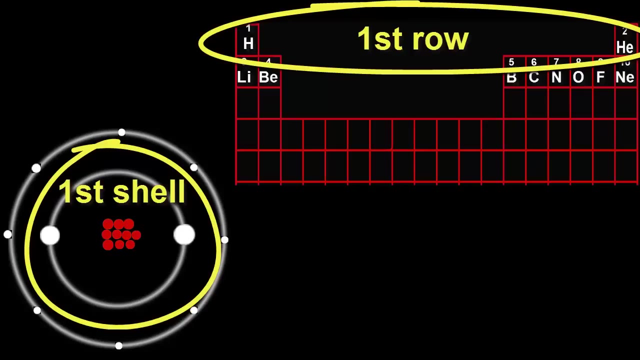 show up on the periodic table. Did you spot the connection between shells and rows? When we filled the first electron shell, we also filled the first row of the periodic table. The first shell takes two electrons before it becomes full and the first row takes two elements. 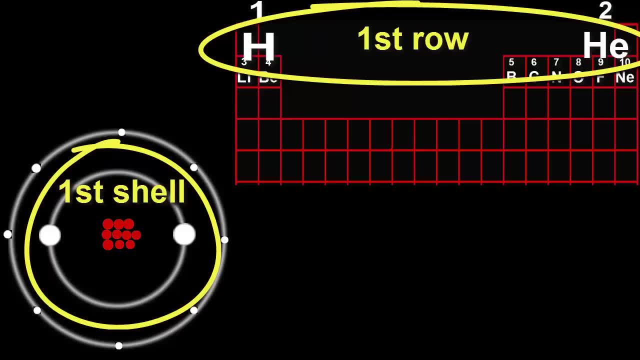 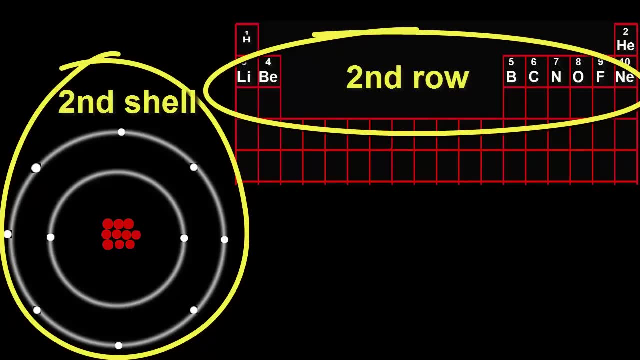 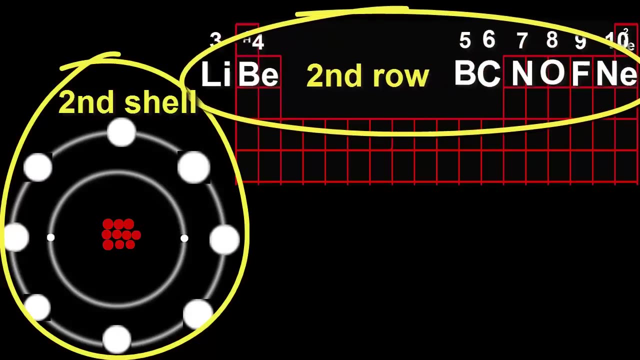 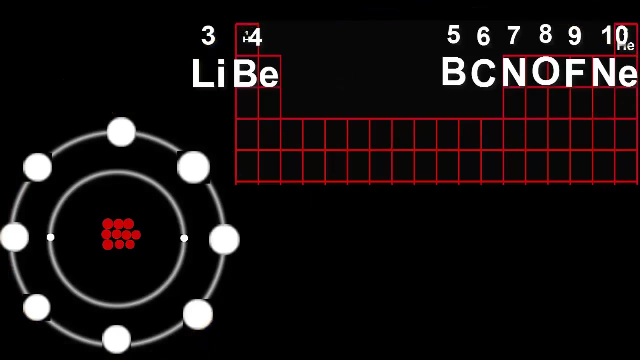 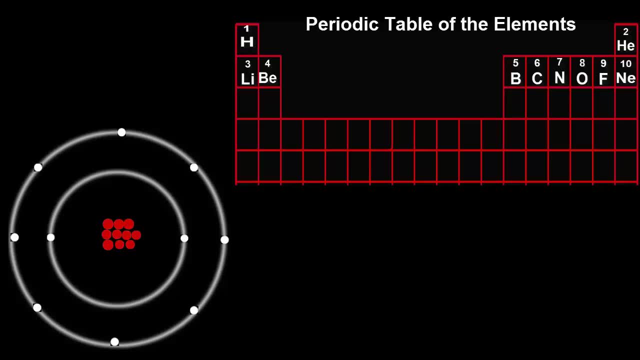 According to our new theory, the number of electrons that it takes to fill the third shell is the same as the number of elements In the third row of the periodic table. Let's count them: One, two, three, four, five, six, seven, eight. 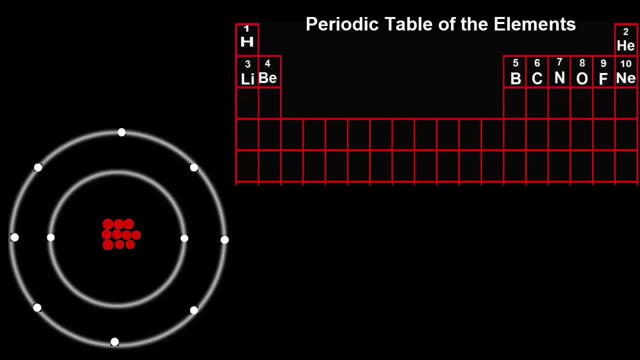 The third shell can take eight electrons, same as the second shell. While we're at it, let's count the fourth row: One, two, three, four, five, six, seven, eight, nine, ten, eleven, twelve, eight. 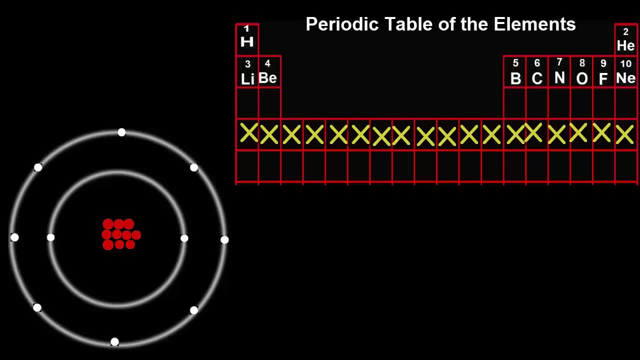 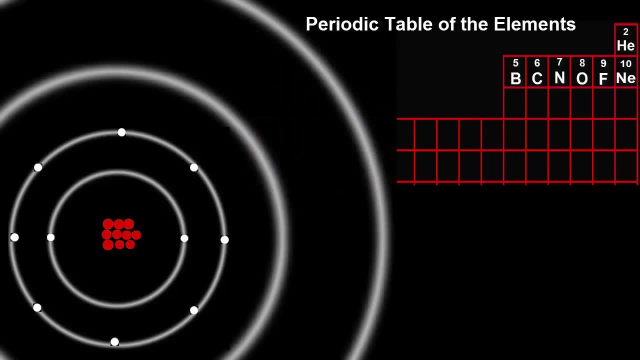 So it must take eighteen electrons to fill the fourth shell. Does this agree with the experiment? Yes, it does. Scientists have measured the number of electrons in each shell and this agrees with our answers: Two in the first shell, eight in the second, eight in the third and eighteen in the fourth shell. 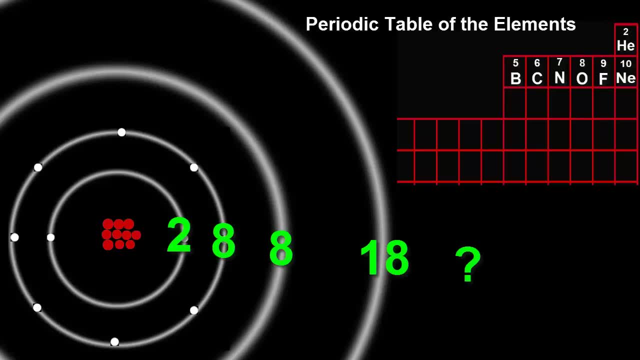 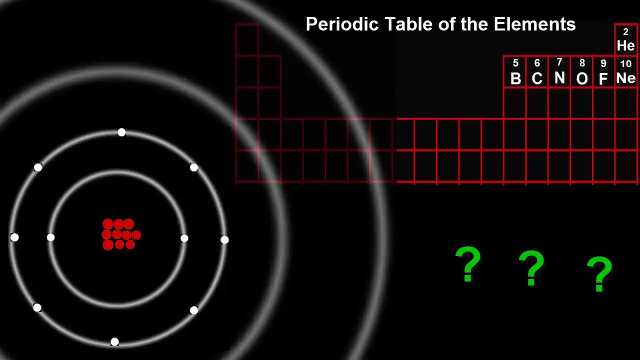 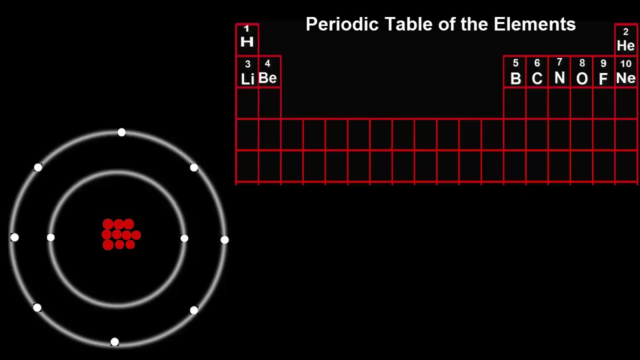 So how many electrons can the fourth shell fill, And what can the fifth, sixth and seventh shells take? See if you can work it out. In the next video we will see how the electrons in the outer shell are the most important ones. 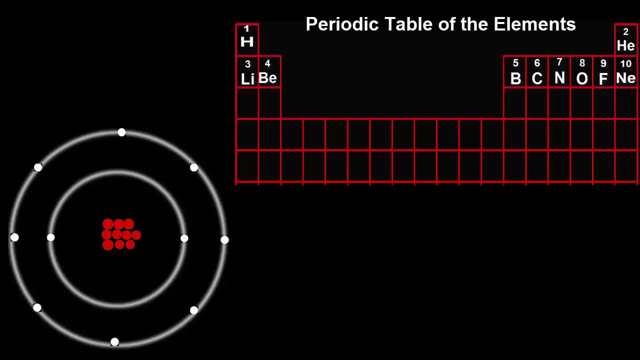 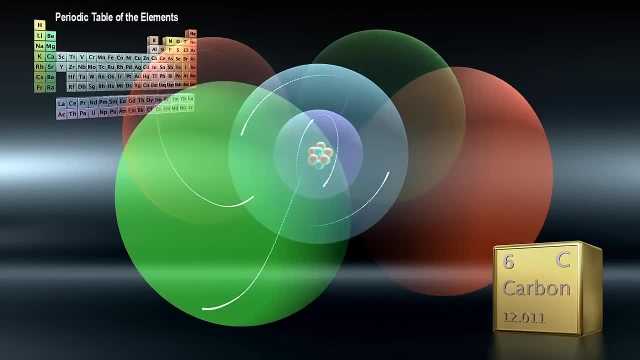 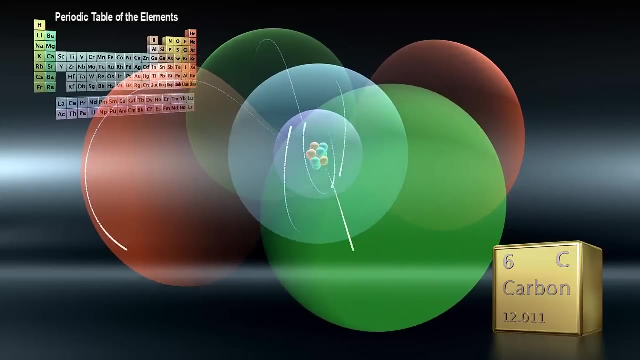 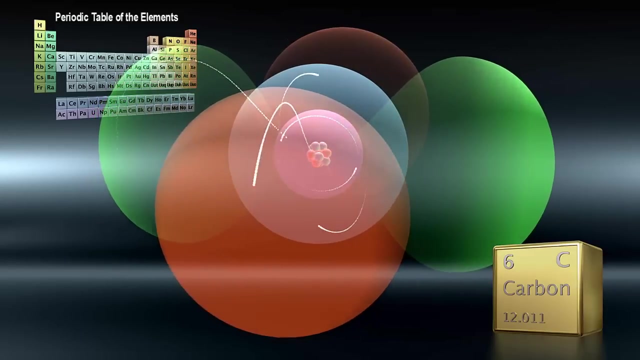 They tell the element how to behave, That is, what properties it will have, such as color hardness, electrical conductivity and so on. They also tell the atom how it will join with other atoms and how many to join with. The outer electrons are called the valence electrons and they're really cool.